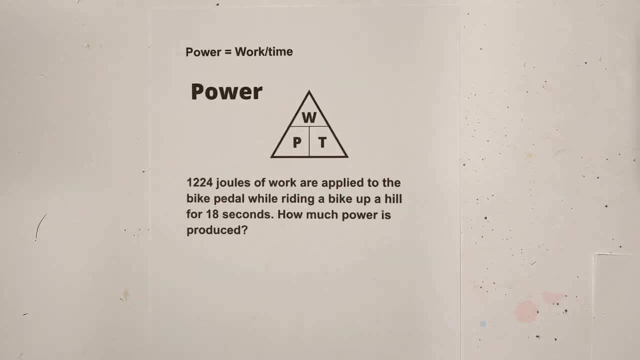 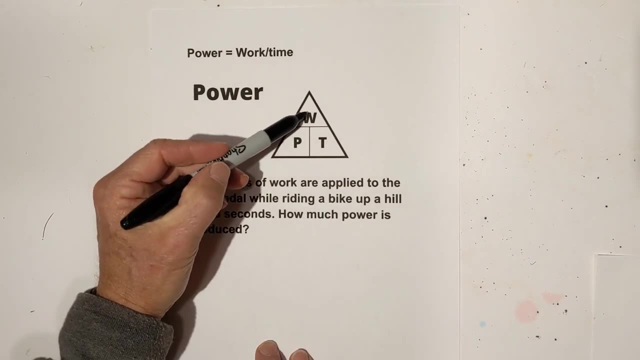 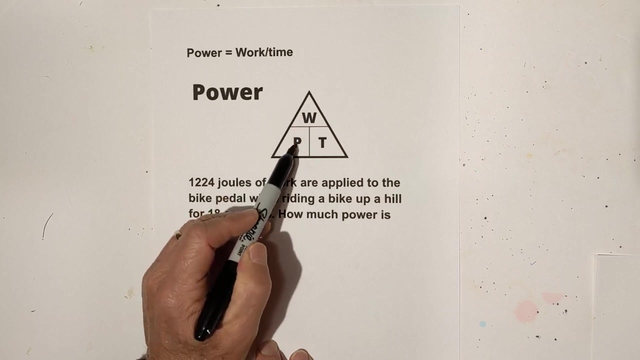 Welcome to MooMooMath and Science. In this video, let's figure out how to calculate power, and the formula for power is work divided by time. Now you can use this triangle to help you figure out other things like power, time and work, For example. if you need power, it's. 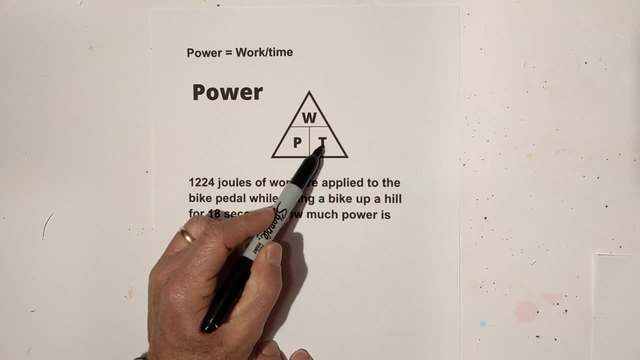 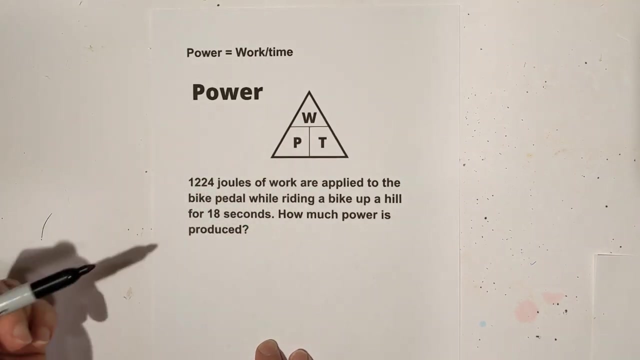 work divided by time. If you need how long you need to apply something, it is work divided by power and then, if you would like to know how much work is produced, it's power times time, and I'll work an example of each of these. So let's get started. Okay, we have 1224 joules of work are 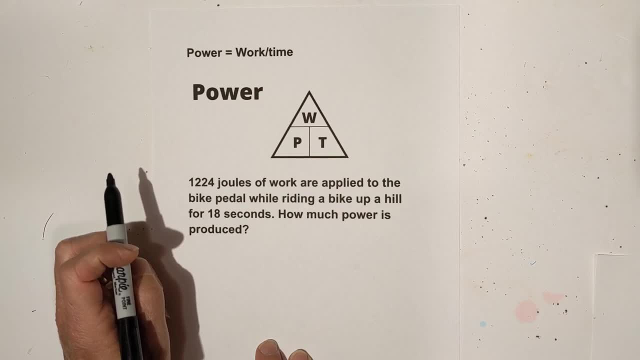 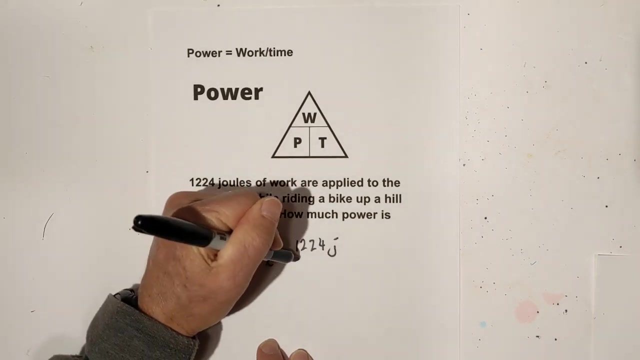 applied to the bike pedal while riding a bike up a hill for 18 seconds. How much power is produced? Remember, power is work over time. So now let's start plugging in some numbers. We have 1224 joules And that is applied for 18 seconds. Okay when that's a messy j, by the way. Okay when you take. 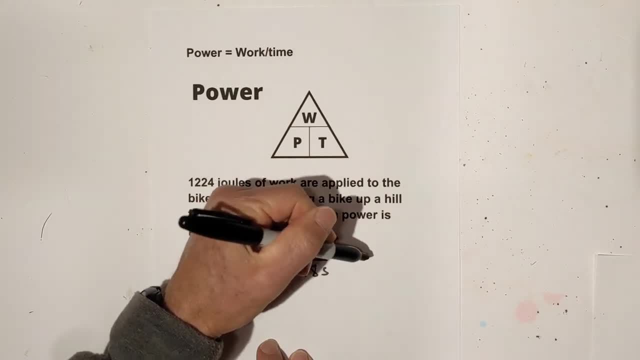 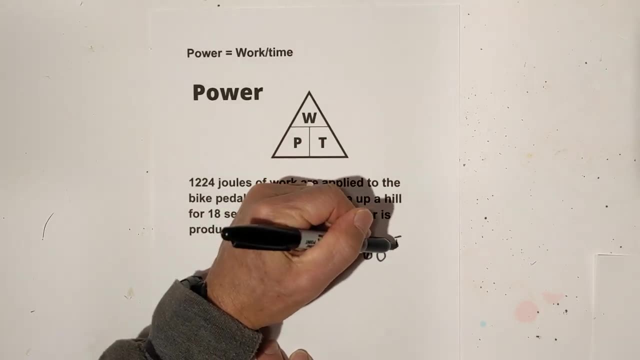 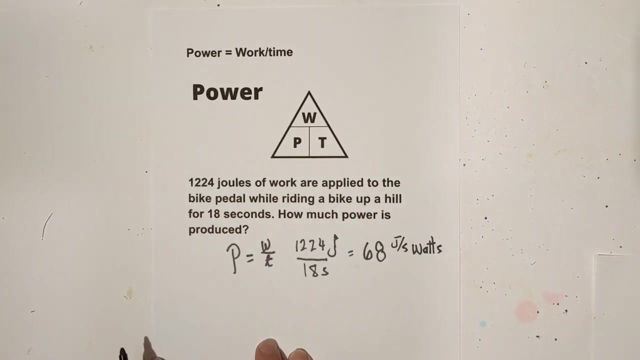 1224 divided by 18, that gives you 68.. But now we've got to make sure we get the correct units of measure. We have joules divided by seconds, which is a watt, So we have 68 watts of power is produced. 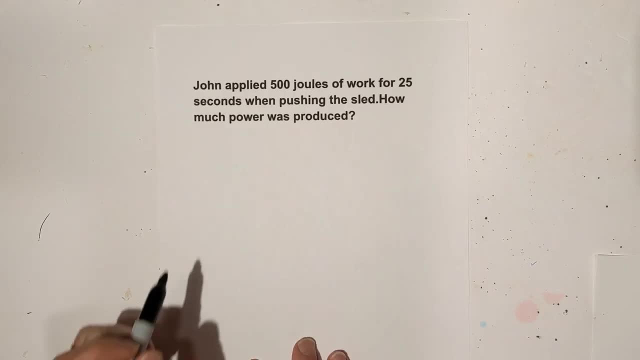 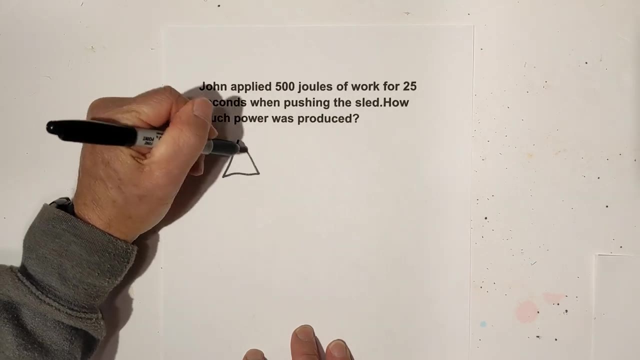 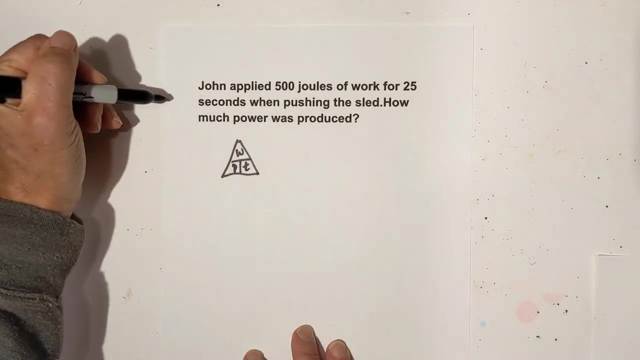 Let's look at another example. Okay, this time we have. John applied 500 joules of work for 25 seconds when pushing the sled. How much power was produced? Again, I'm going to draw this. You don't have to draw this chart each time, but I just want to emphasize this. And so we are looking for power. 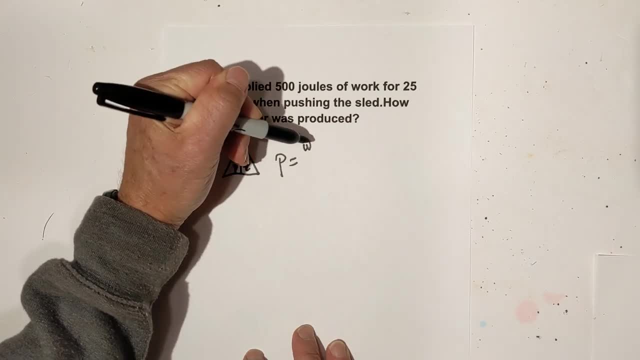 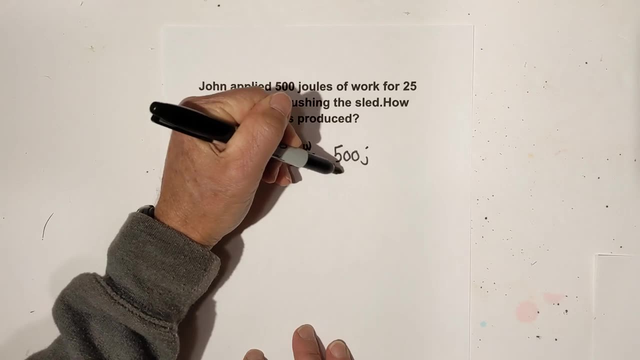 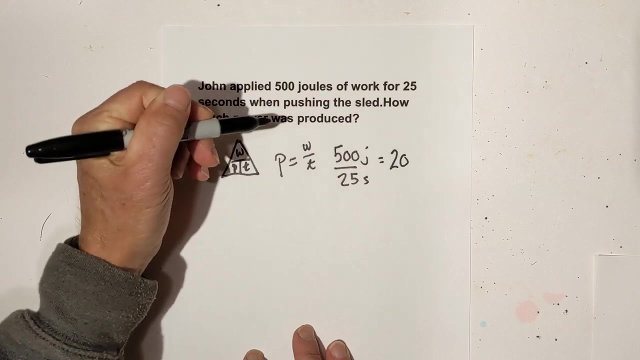 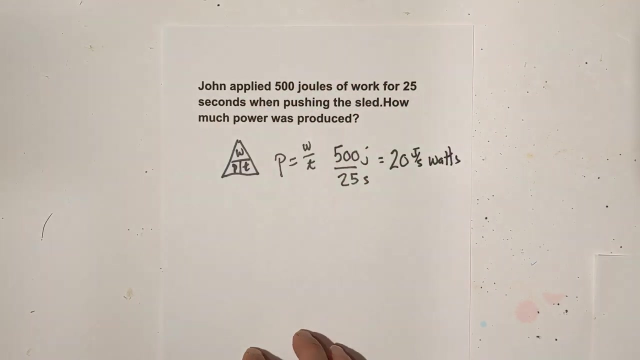 and power is equal to work over time. So we have 500 joules of work, and that was for 25 seconds. When you divide 500 by 25, that gives you a second. Remember we have joules per second. which is what? So it is 20 watts. Now we're going. 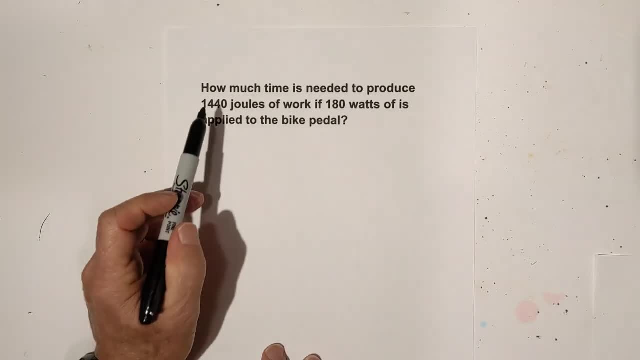 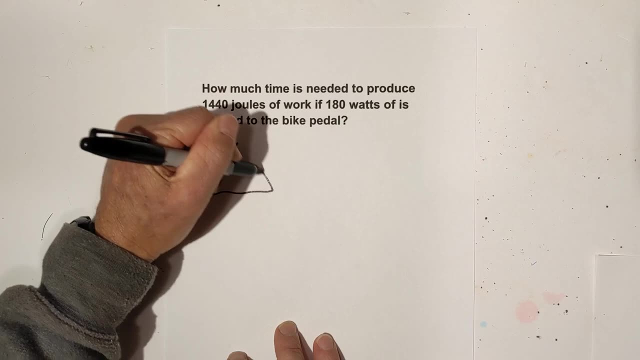 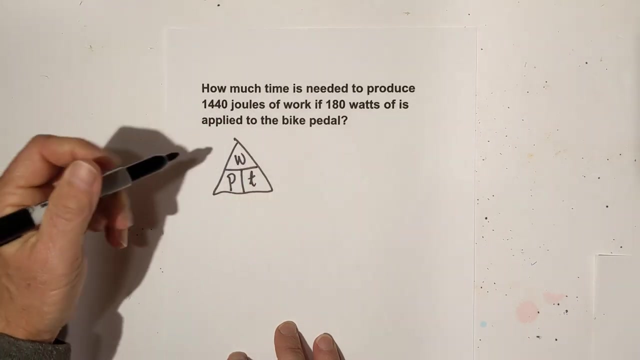 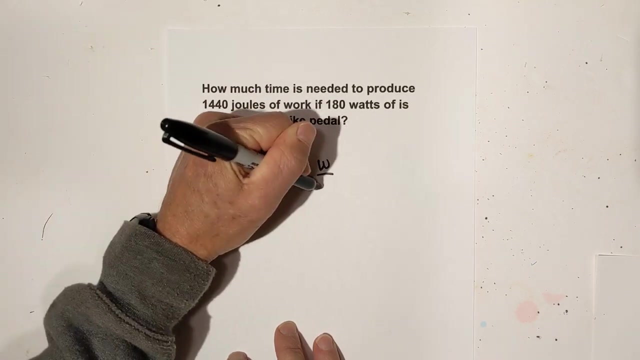 to do two that are slightly different. Okay, and this one is how much time is needed to produce 1400 joules of work if 180 watts is applied to a bike peddle. So let's look at our triangle again: Work, work, power time. this time we are looking for time, and time is work over power, work over. 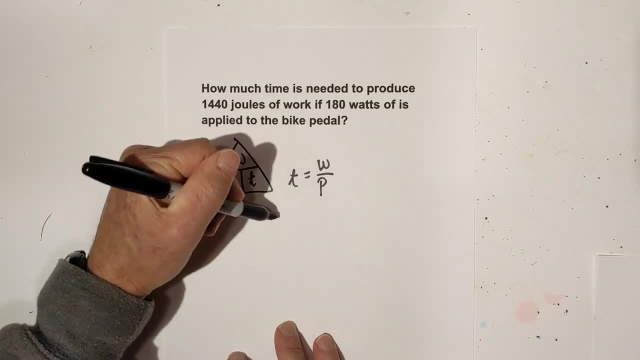 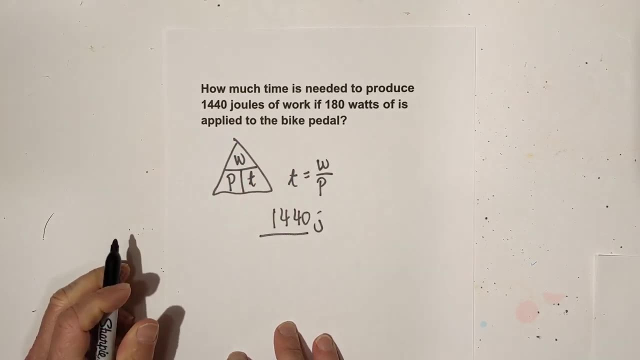 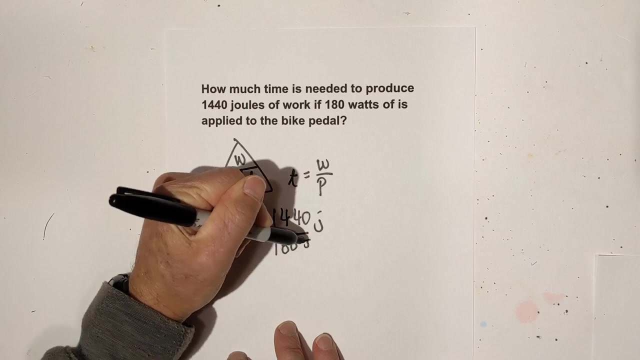 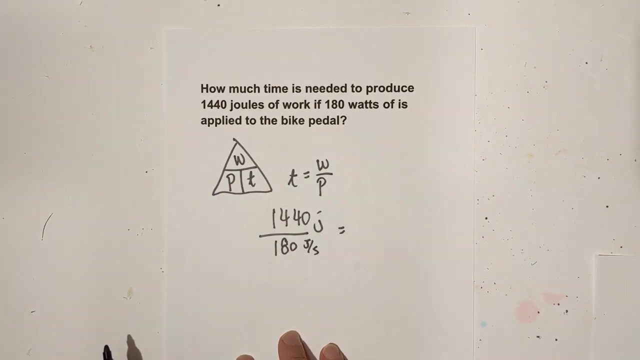 power. let's see how much work we have. we have 1440 joules of work and our power is 180 watts. now I am going to write the 180 watts as joules over seconds. so when we divide 1440 by 180 watts, that is 8. so now lets look at the units of measure. we have joules. I am going 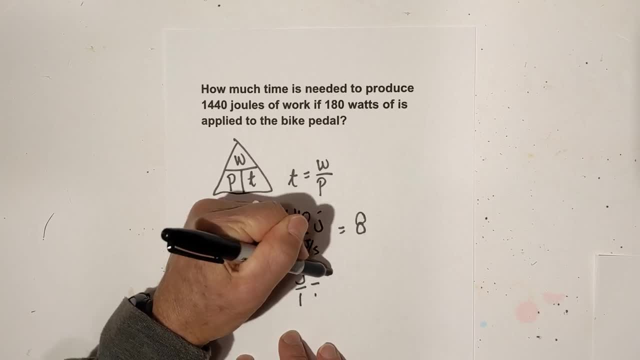 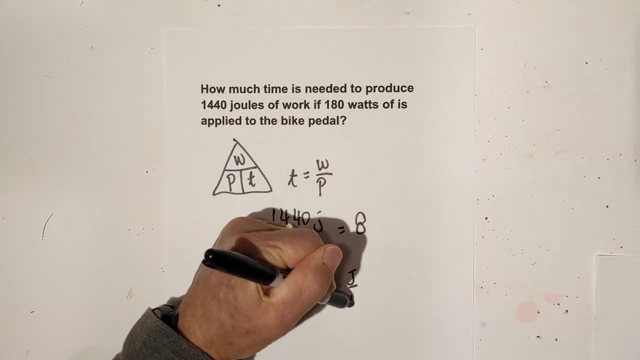 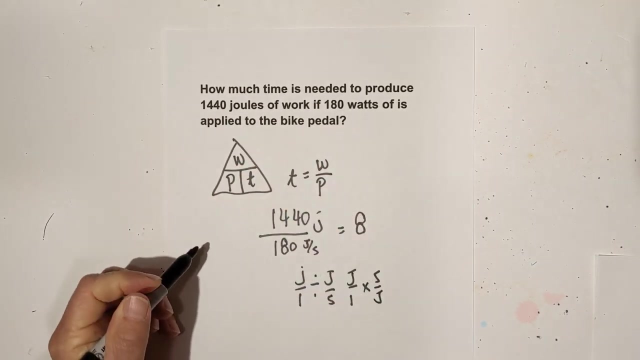 to write joules over one, divided by joules over seconds. ok, When we divide, we're going to keep, we're going to change, we're going to flip, okay. And so now what happens is is the joules cancel and we're left with seconds, okay. 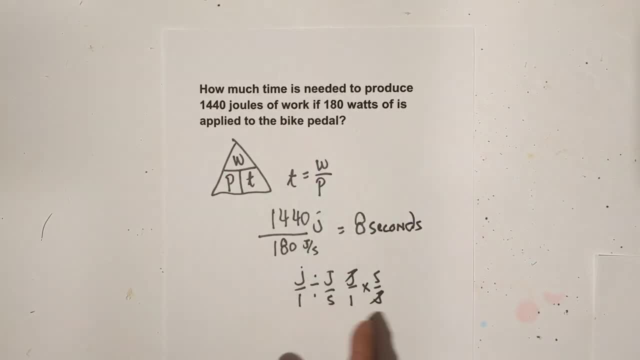 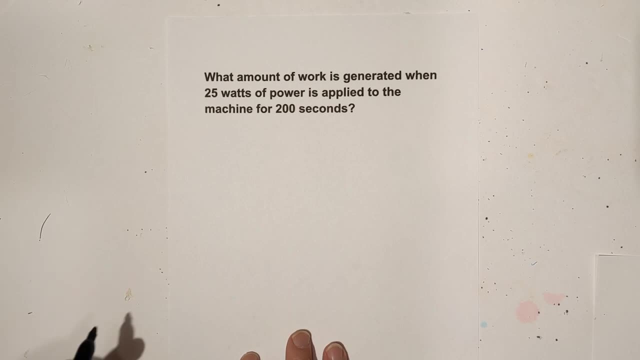 I just wanted you to be aware the units of measure and what is taking place there. Let's look at our final example. Okay, for our final example. what amount of work is generated when 25 watts of power is applied to the machine for 20 seconds? 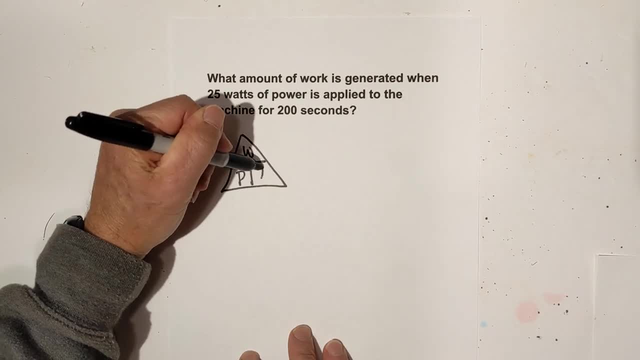 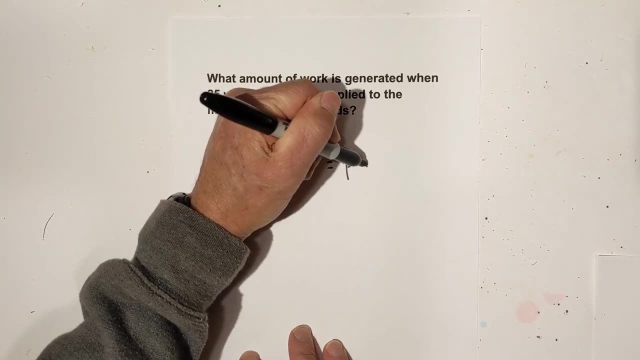 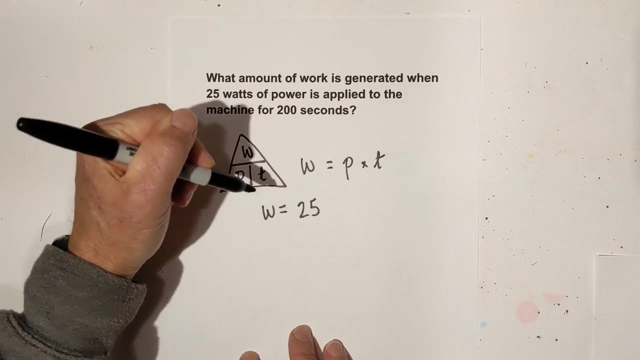 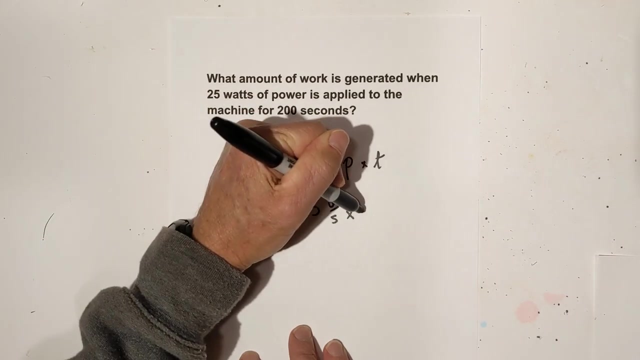 So watch, we have work power time, We're looking for work and that is going to be equal to power times time. It says we have 25 watts of power and remember watts is joules over seconds times 200 seconds. okay, 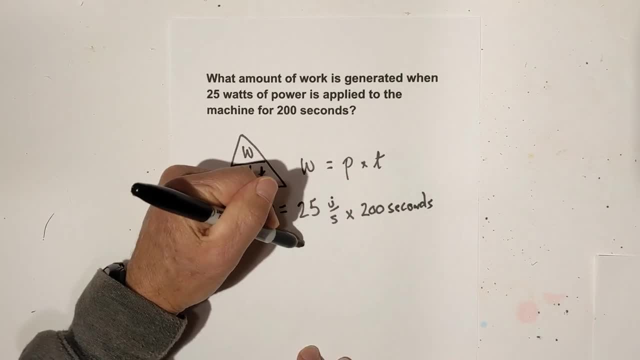 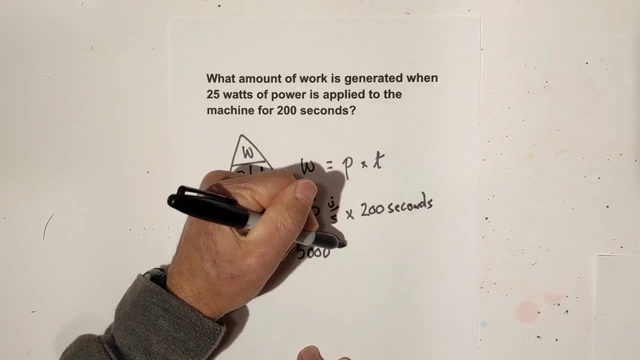 So now, when we multiply this 25 times 200 seconds is 5,000,. okay, And let's see what we have with our units. We have joules over second times seconds and I'm going to place it over one.